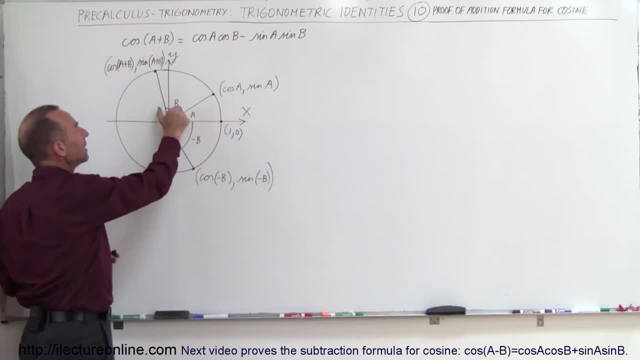 a unit circle right here and let's say we have the angle a and the angle b and also the angle minus b. So we have one, two, three, four points here on the unit circle. We have the point right here, We have the point right there which is defined by the cosine of a and the sine of a. 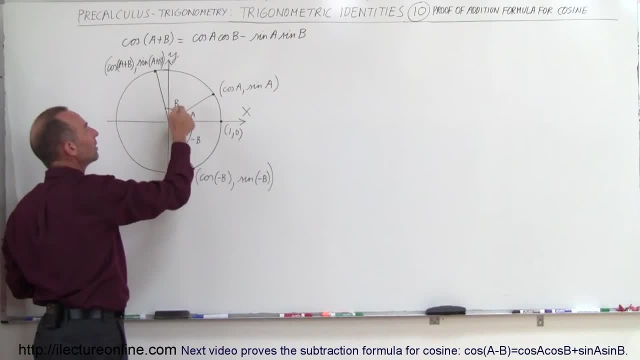 as the coordinates of that point, Since if we add a plus b together, that means that here the coordinates of this is the cosine of a plus b and the sine of a plus b, simply adding those two together. And since there's a negative angle right here, this would be the cosine of negative b. 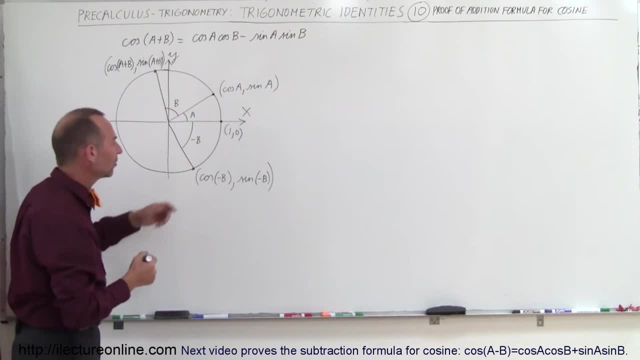 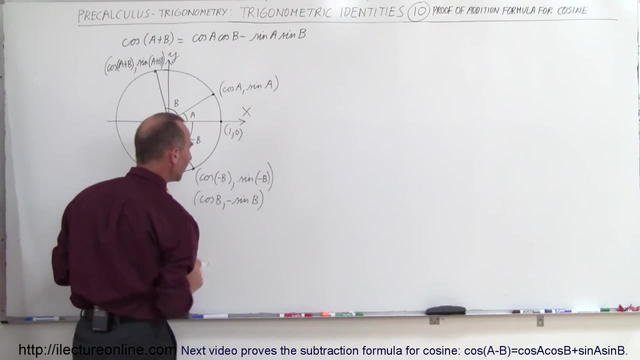 and the sine of negative b. Of course, we also know that this can also be written as the cosine of b and minus the sine of b, like that, Because the cosine of a negative angle is the same as the cosine of a positive angle and with the 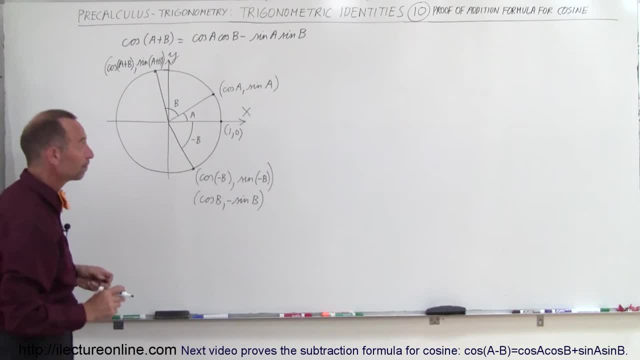 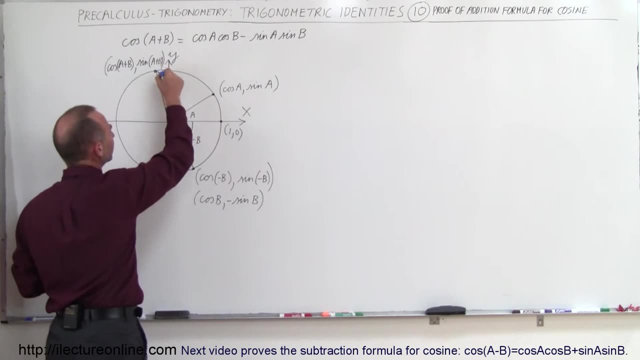 sine, we simply have to put a negative in front of it to set it equal to each other. Now, what we're going to do is we're going to draw a chord. We're going to draw a line from this point to this point and a line from this point to this point, And notice that, since the angle a plus b here is the 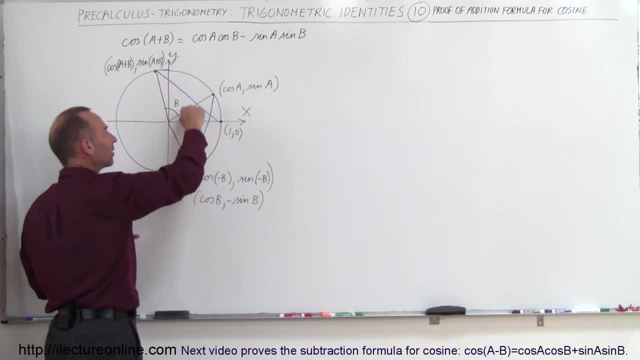 same as the angle a plus the negative b right here. this angle here must be the same as this angle there. That means the length of the angle is the same as the angle b right here. And since the angle a plus b is the same as the angle b, the length of those two chords must be the same. 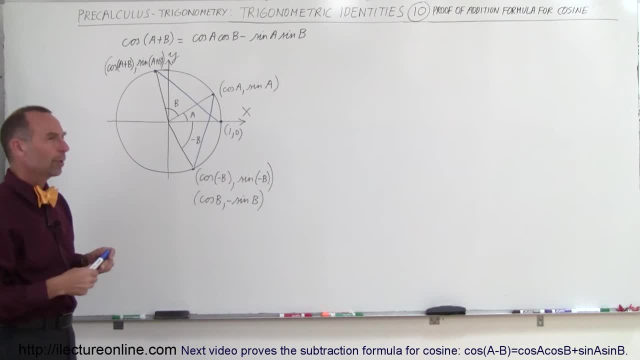 And we can find the length of those chords by using the distance formula. Remember that if we have something like this on the x? y axis, two points of the x? y axis, and we connect them with a line, and this is x1, y1 and this is x2- y2, we can find the distance. d is equal to the square. 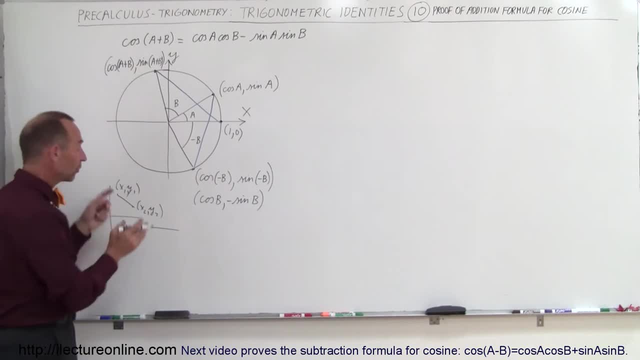 root of the sums of the squares of the difference between the x and the y values of those two points. This is x2 minus x1 squared plus y2 minus y1 squared. We're going to use the same principle here, instead of using x1 and x2, y1 and y2.. We're going to find the coordinate points. 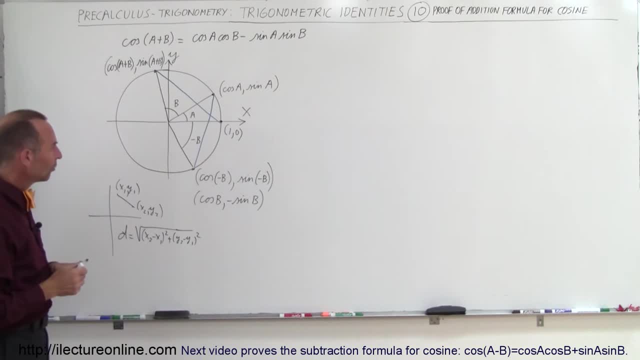 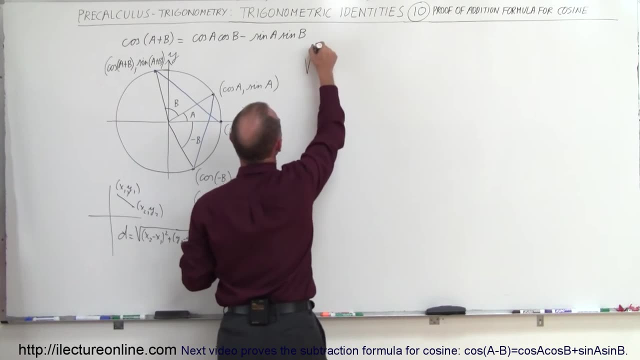 of the points here. All right, so let's find the distance of this line right here. So that means that the line one that would be equal to the square root of the difference in the x value squared, So it's the x value squared, and so on. so there's the x value squared, There's the x value squared. So there's the x values squared. So there's the x values squared. So there's the x values squared. So that's how we can make it, You. so that's how you can make it, You. 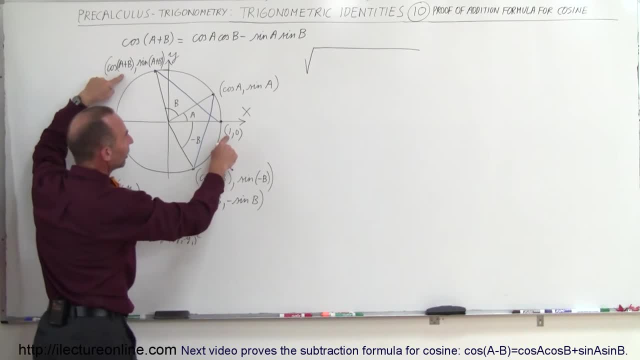 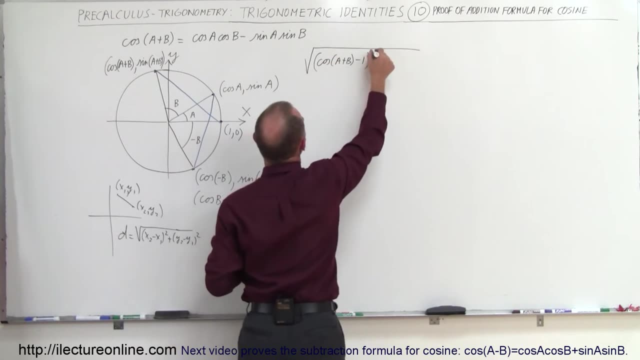 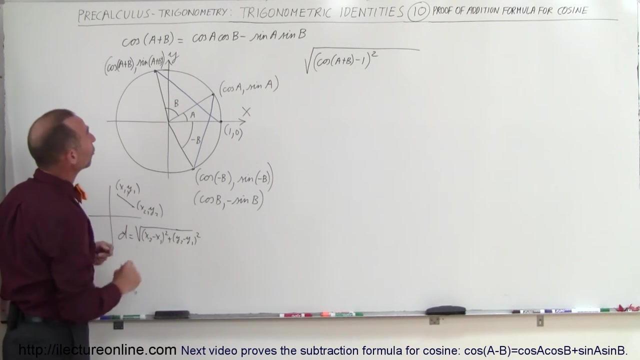 cos a plus b and there's the x value right there one. so we take the cosine of a plus b minus one quantity squared. so that's the same thing as what i have over there. i have the difference in the x values quantity squared, and i add to that the difference of the y value. so 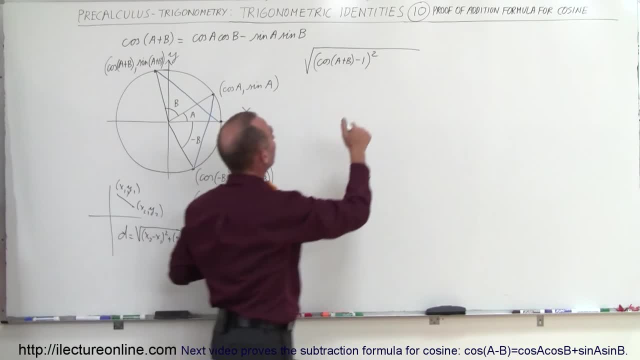 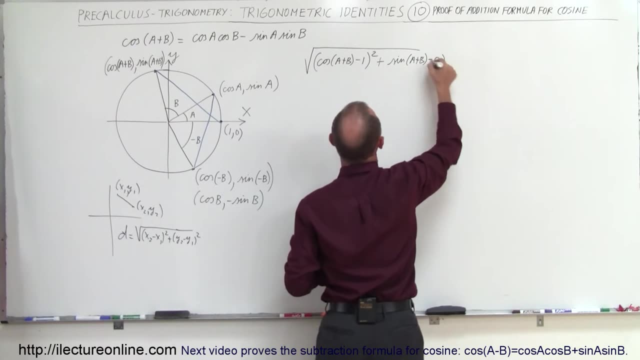 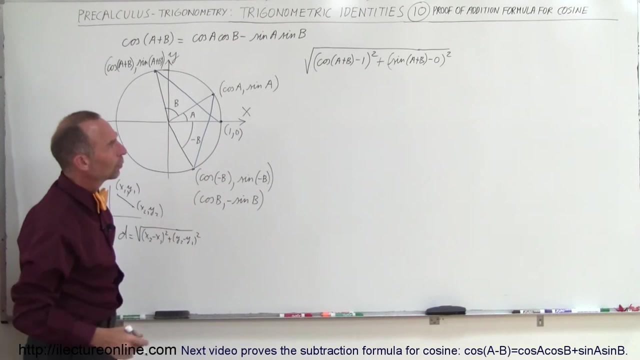 it would be this minus this right here, so that would be plus. we have the sine of a plus b minus zero, quantity squared. of course we don't have to write minus zero, but i just did so to make it visible as to what we're doing here. so that would be the distance for this chord, and 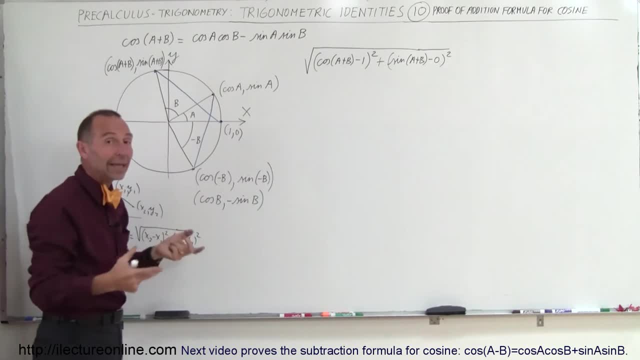 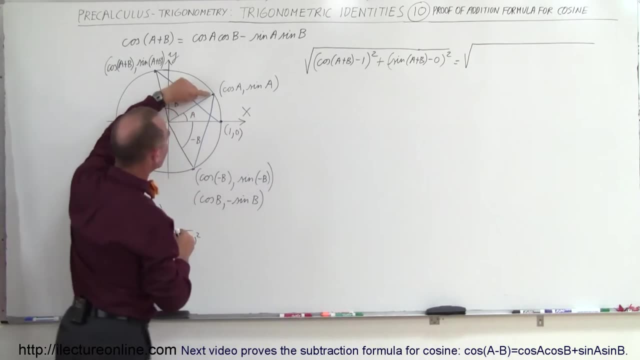 i'm going to take the distance to this chord and since i know that they must be of equal length, i set them equal to each other. so this is equal to the square root of the difference in the x values between these two right here. so that would be the cosine of a minus the cosine of b, quantity squared. 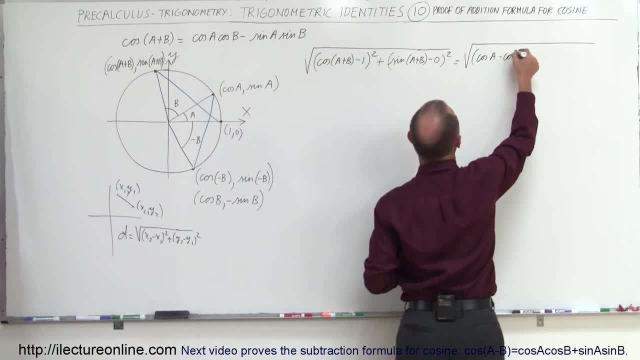 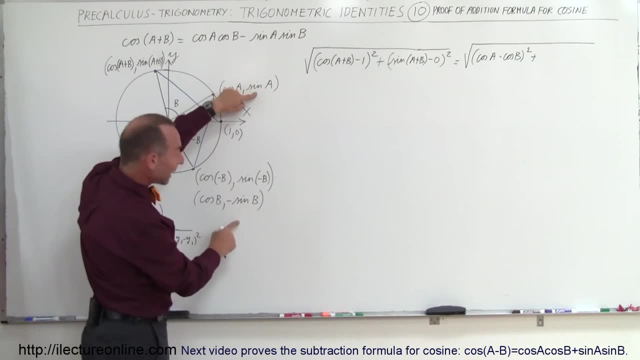 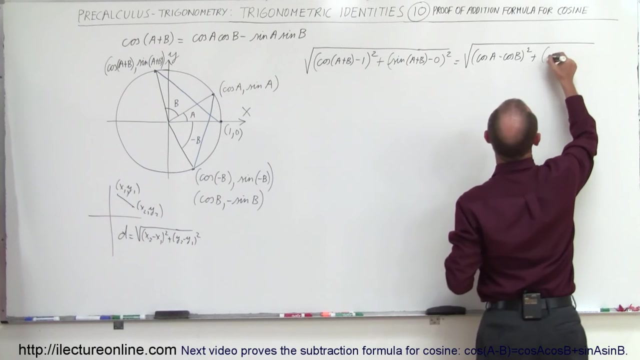 so that would be the cosine of a, you minus the cosine of b, quantity squared plus the difference in the y values, and that would be the sine of a minus minus the sine of b. so negative times, negative, makes that a positive. so sine of a plus sine of b. so it would be sine of a plus sine of b, quantity squared. 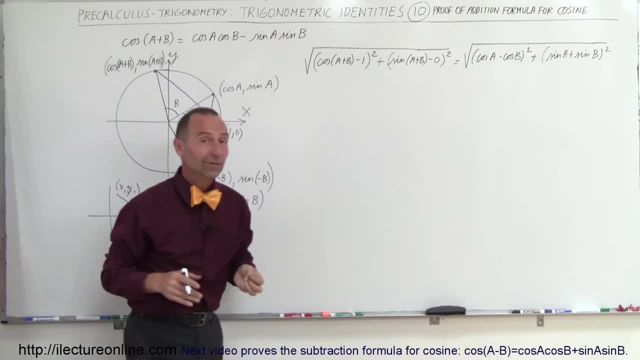 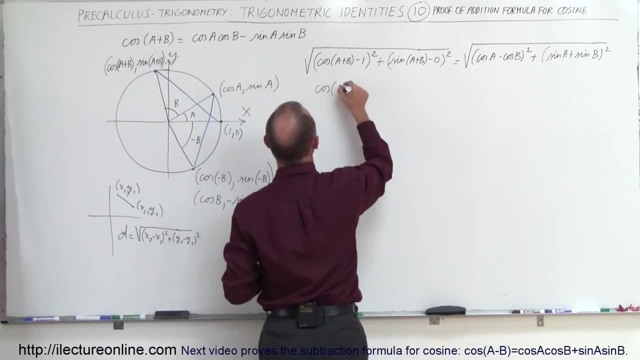 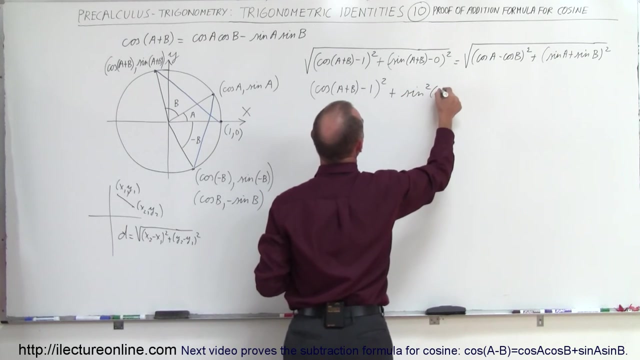 So now I have the two lengths of those two chords set equal to each other, I can now simply square both sides to get rid of the radical. so I can write this now: as the cosine of a plus b minus one squared plus the sine squared of a plus b is equal to. I have the cosine. 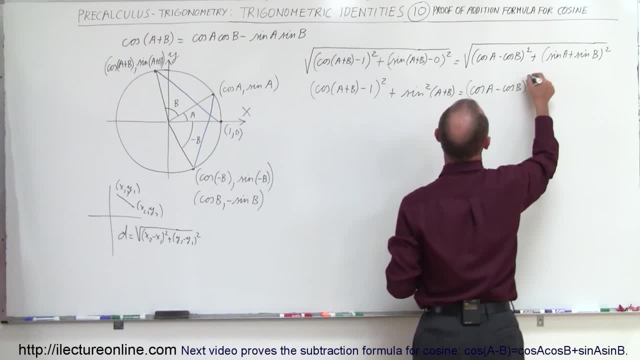 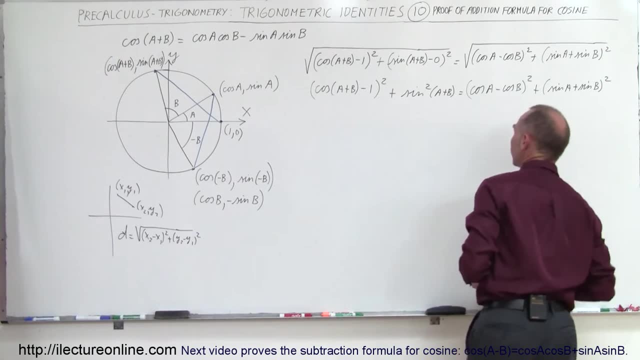 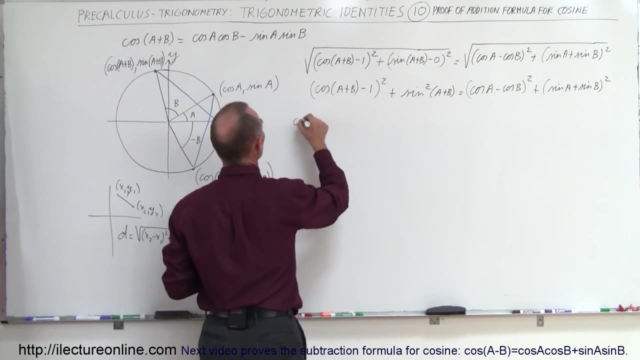 of a minus the cosine of b, quantity squared, plus the sine of a plus the sine of b, quantity squared. So now what we need to do is simply Square everything out. see what we get. so when we square everything, we get the following: we get the cosine squared of a plus b. these two multiply times two, so minus two times. 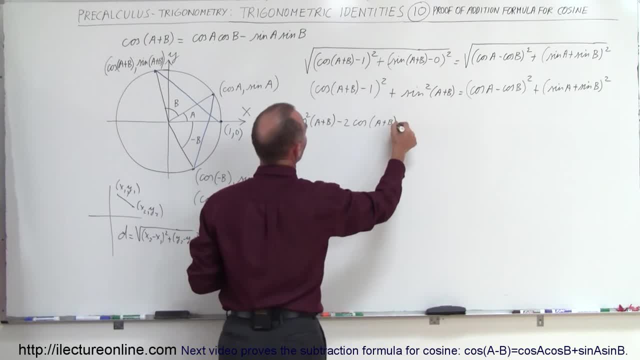 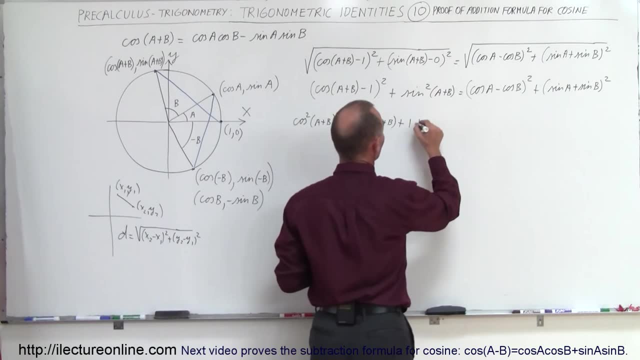 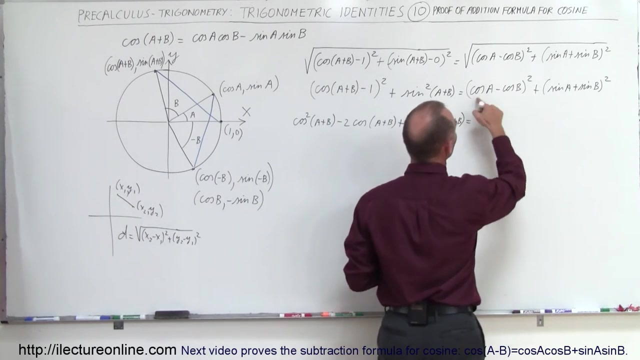 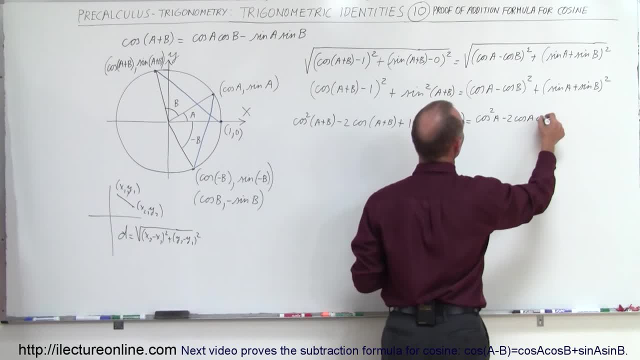 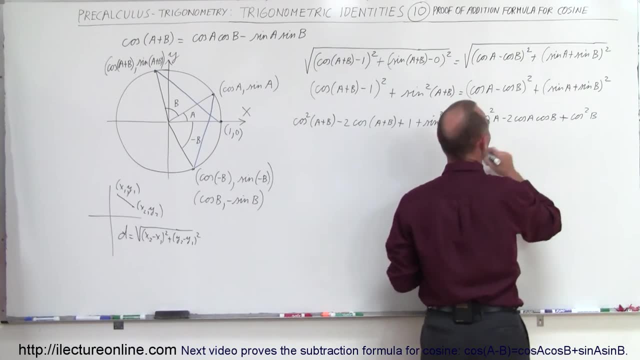 squared of a minus two times of cosine a, cosine b plus the cosine squared of b plus the amount of room. I just continue like this. multiply this out, so we have the sine squared of a plus two times the cosine, two times the sine, a times the sine of b, plus one squared. 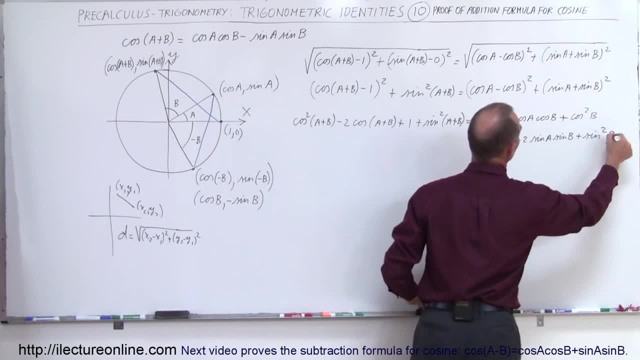 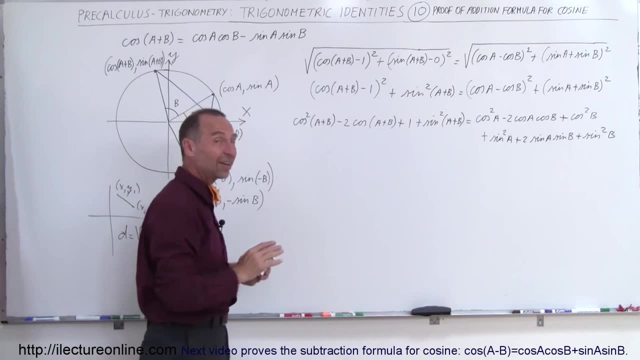 plus the sine square of b. All right, now we have a big mess. Apparently it looks like a big mess, but don't panic here because, as you can see, there's a lot of simplification here. We have the cosine square of a plus b. 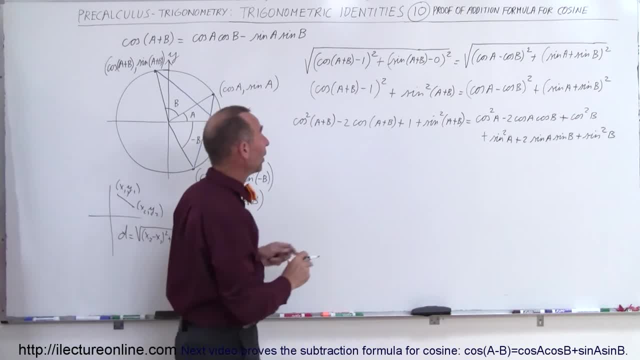 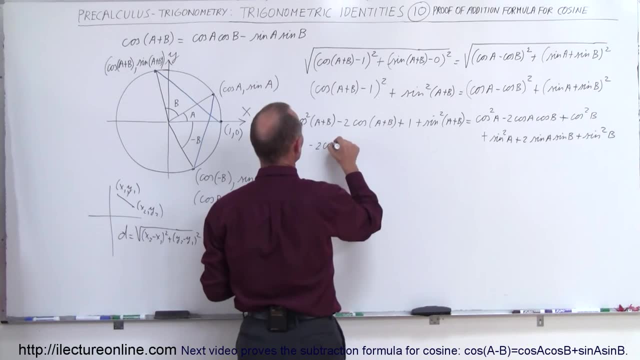 plus the sine square of a plus b. We know that that adds up to 1, so we can just add these two together and add that to this. That gives us 2 on the left side. so we end up with a minus 2 times the cosine of a plus b. 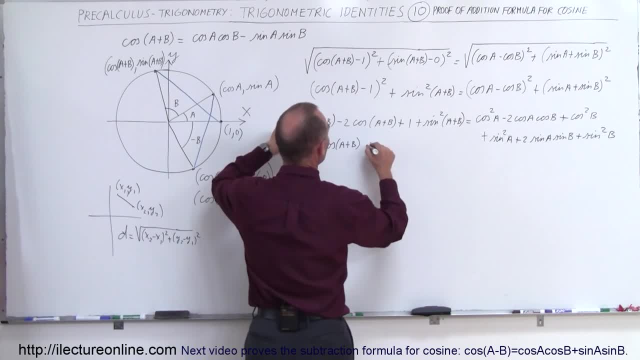 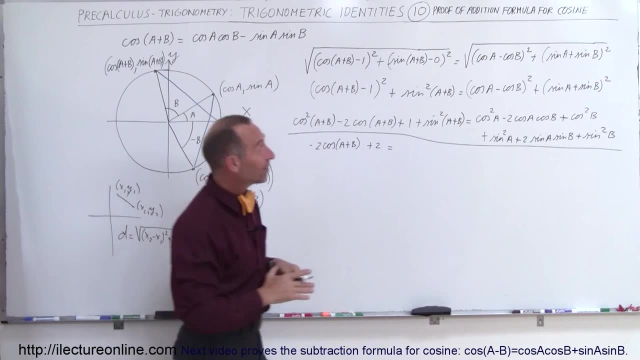 plus 1 plus another 1, so that would be plus 2 equals- and let me draw a big line here so I don't get that confused there. Now on the right side, notice- we have a cosine square of a and a sine square of a. 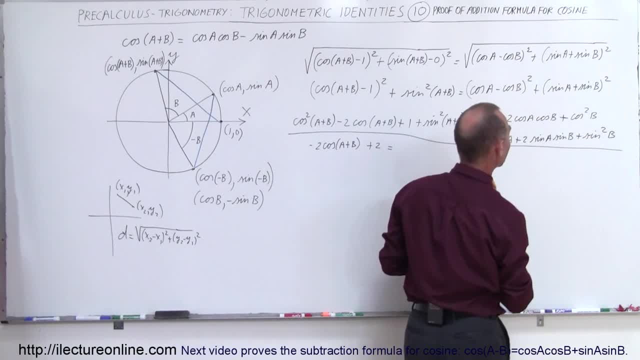 so add these two together, that gives me 1.. And do I have anything else like that? A cosine square of b plus a sine square of b, so these combine to 1 and those combine to 1, so let me just draw little circles around it. 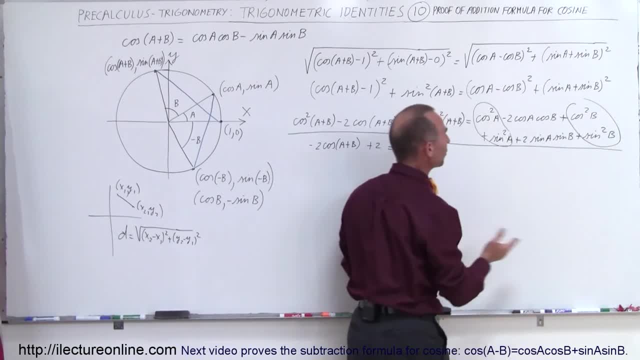 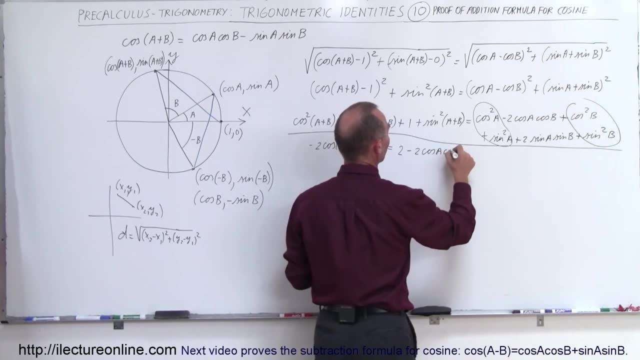 so that combines and becomes 1,. this combines and becomes 1,, so that would be 2, so on the right side I end up with 2 minus 2 times the cosine of a, times the cosine of b, plus 2 times the sine of a, times the sine of b. 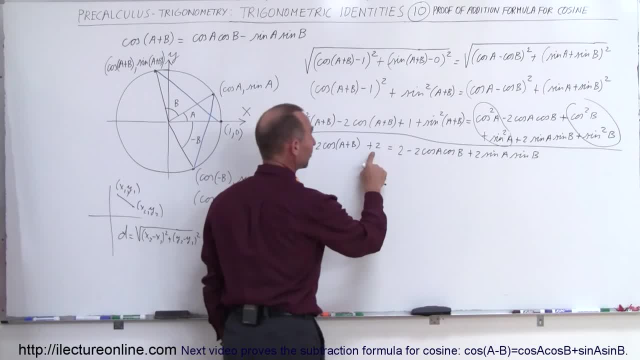 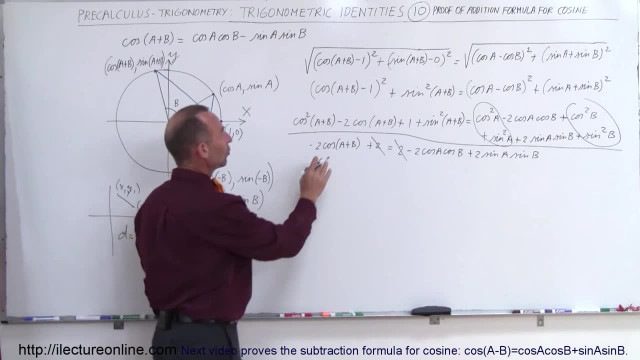 All right. Now notice that we have a plus 2 on the left side and a plus 2 on the right side. so those cancel out. so that's gone, And now I have a cosine of a plus b times a negative 2..